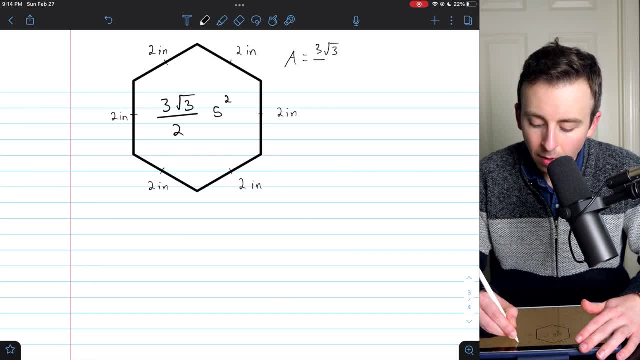 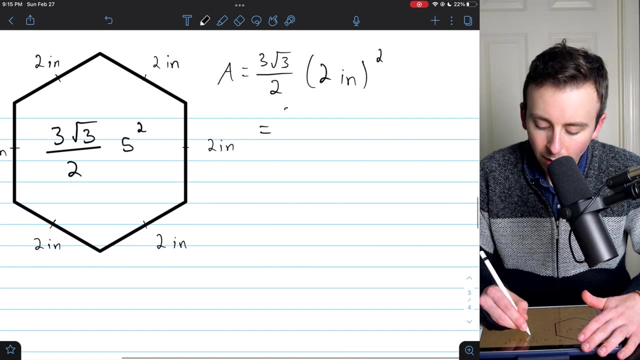 So that's just 3 root 3 over 2.. And then multiply by the side length squared. The side length is 2 inches. So we multiply by side length squared And what's this equal to? Let's go ahead and zoom in a little bit. 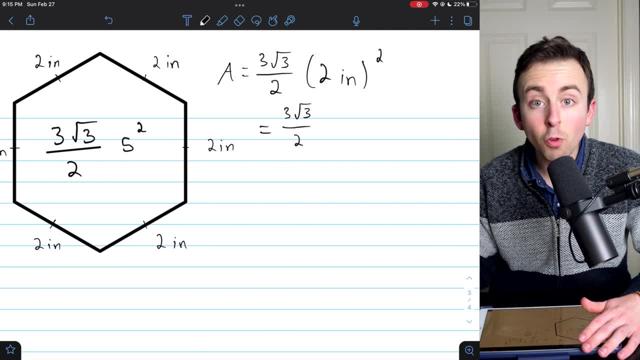 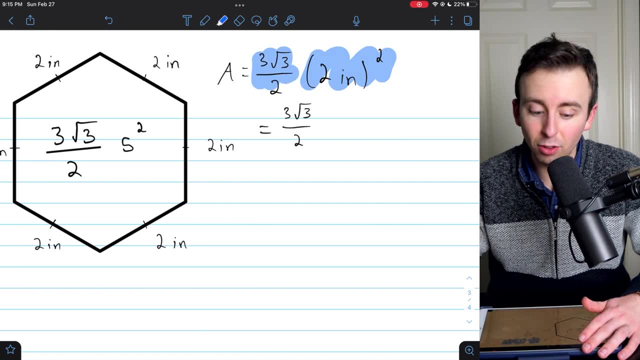 Well, we've just got 3 root 3 over 2.. Remember, it's the side length that's squared, The 3 root 3 over 2, that is not squared. So then, what is 2 inches squared? Well, you've got to remember to square the 2, which gives you 2.. 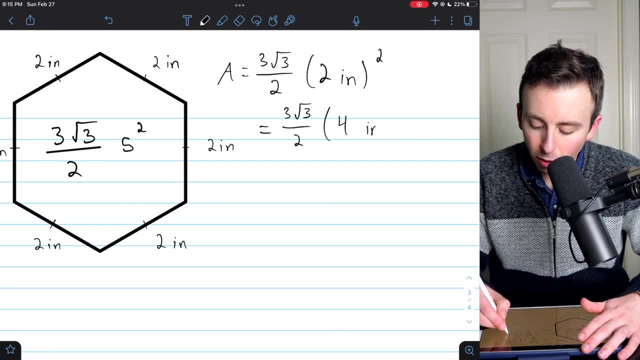 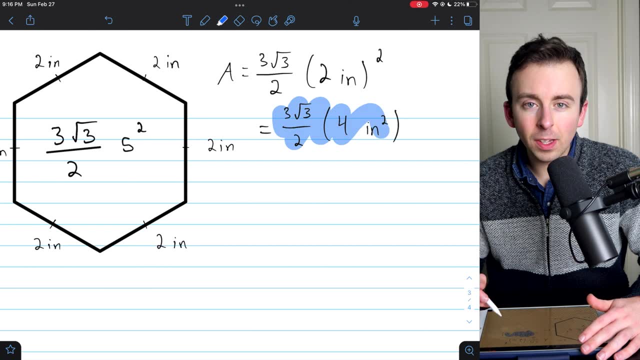 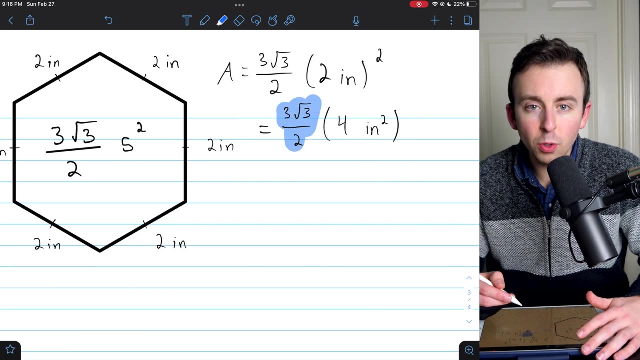 Which gives us 4.. And then we also have to square the inches to give us our proper area units: inches squared. Now can we simplify this at all? Yes, we can. You've got to remember that fractions mean division. 3 root 3 over 2, that means divide by 2.. 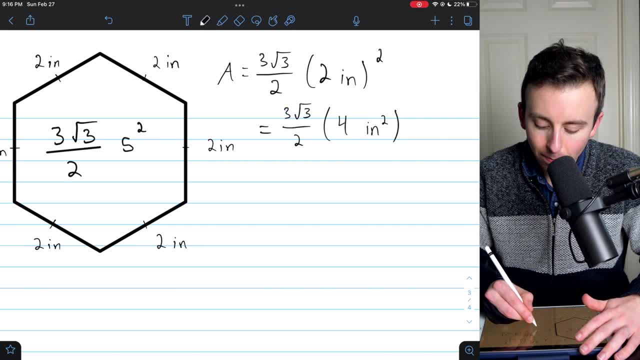 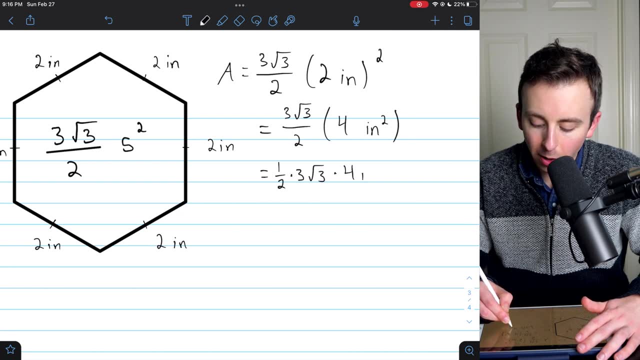 And division is the same as multiplication, right? This is the same as 1 half times 3 root 3 over 2.. Times 4 inches squared And we can do multiplication in whatever order we please. Point is we can take 1 half of 4.. 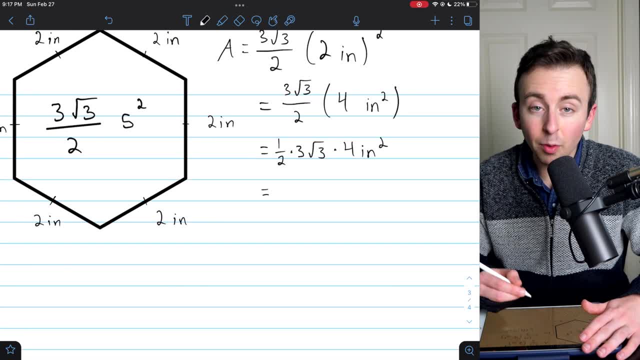 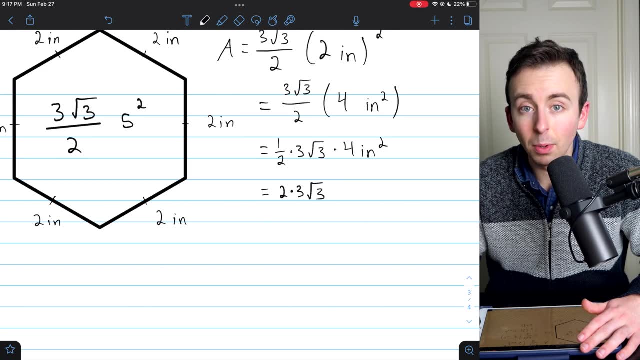 And that's going to simplify this a little bit. Now, 1 half of 4 is just 2.. So we would be left with 2 times 3 root 3.. But 2 times 3 is just 6.. So that's actually 6 root 3.. 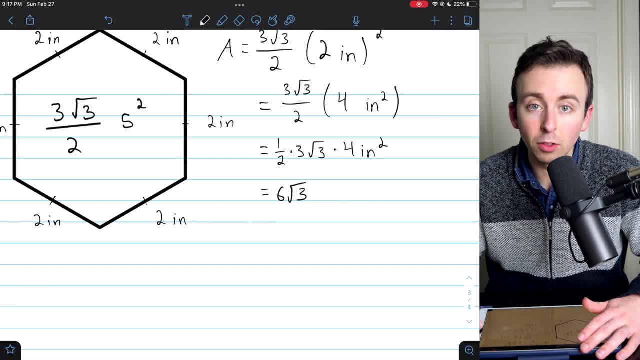 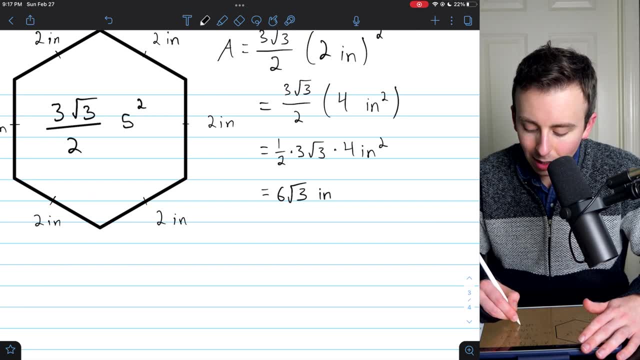 Remember, multiplication is commutative. That's why I've been able to do this. I've been able to swap the order of these things around with no trouble. So we've just got 6 root 3.. And then don't forget our units: inches squared. 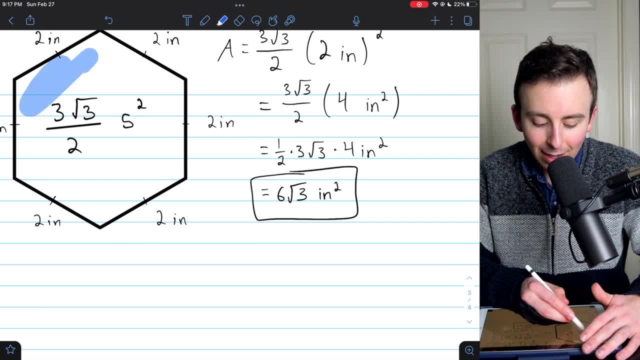 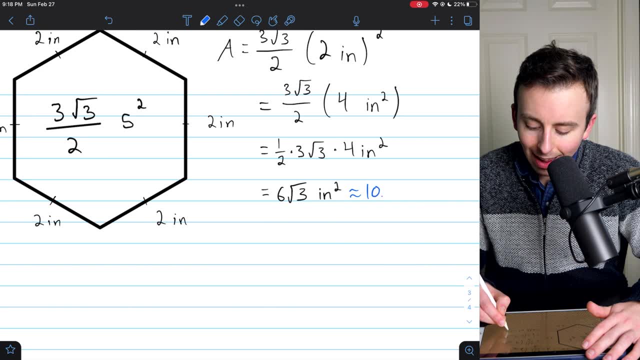 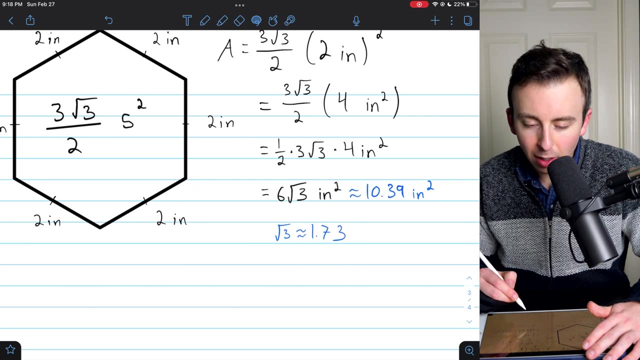 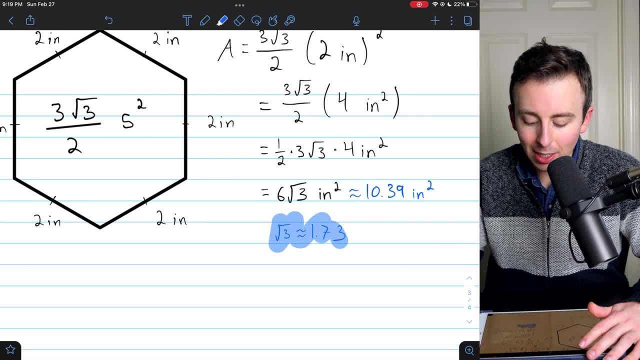 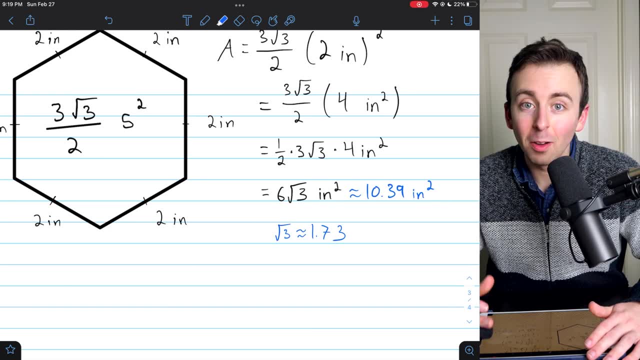 So if you don't have a square root button, you could use that, But really, if you don't have a square root button, what you need is a new calculator. So that's how you calculate the area of a regular hexagon. 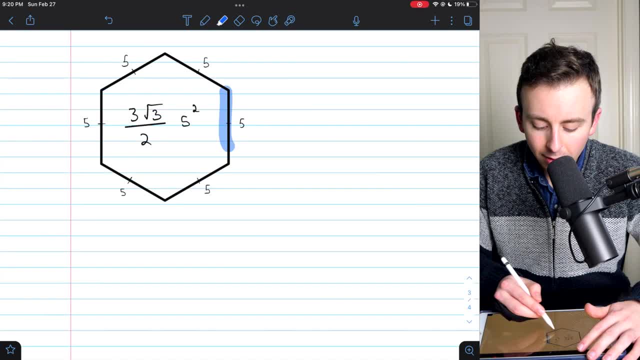 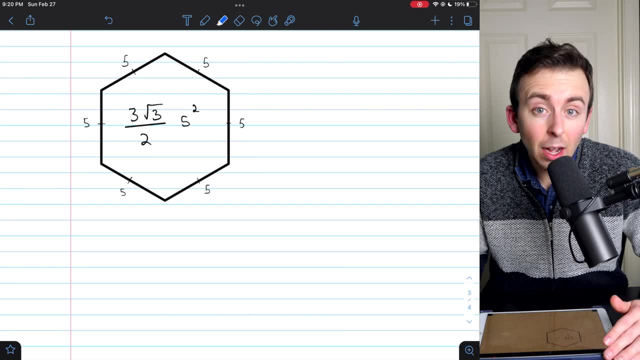 Let's do one more example. Let's suppose we've got a regular hexagon with sides of length 5. What are the units? Well, the units really don't matter, because we're calculating area. The units of area are something like length squared. 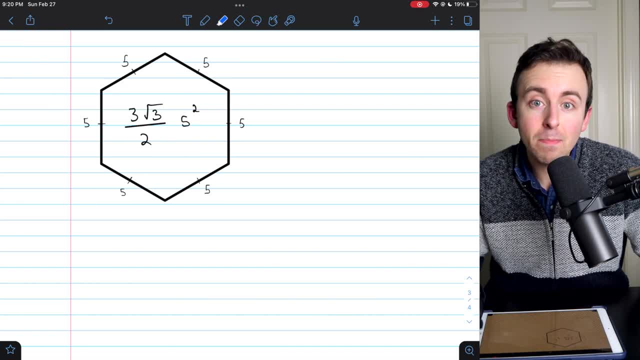 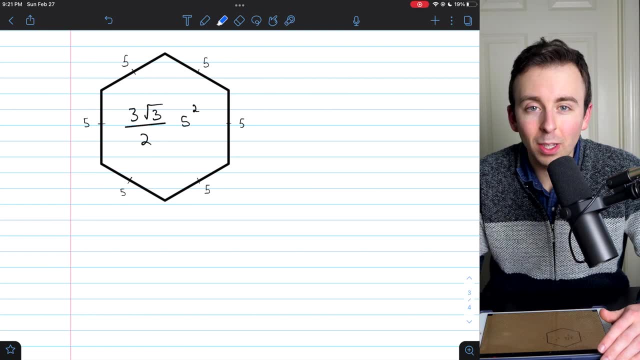 So if your side lengths are in miles, the area is going to be miles squared. If the side length is in meters, the area is going to be meters squared. We really don't have to worry about the units. We know what our final units are going to be. 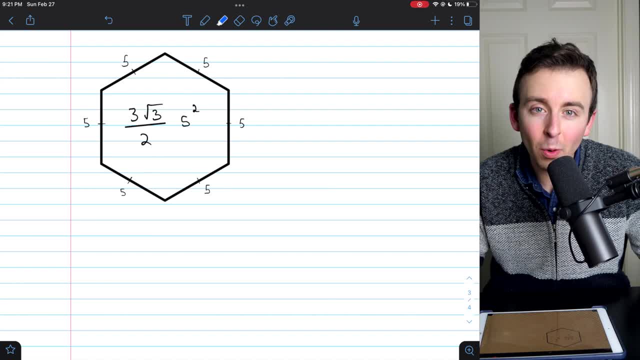 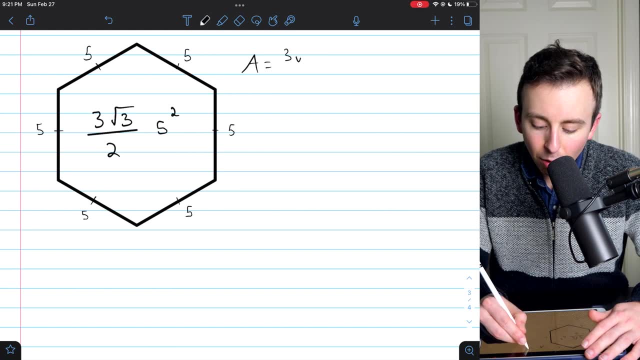 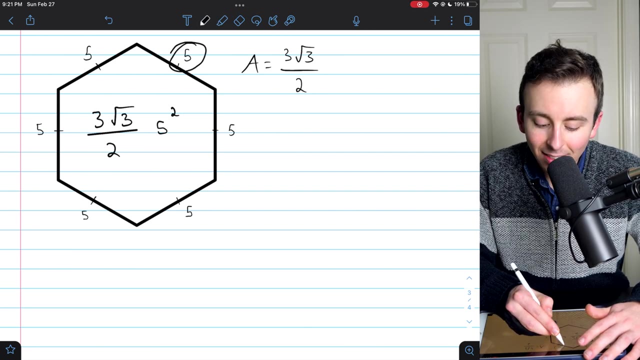 It's just going to be the lengths unit squared, So let's just ignore units and carry on with the calculation. What's the area of the regular hexagon? It's 3 root 3 over 2 times the side length squared, In this case the side length. 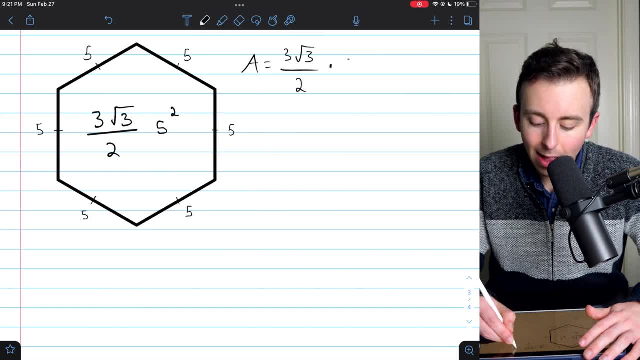 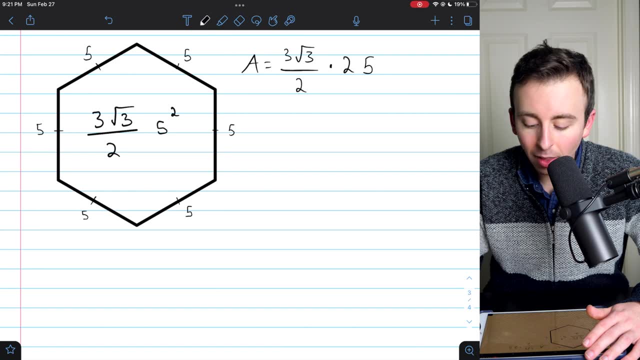 the area of the regular hexagon is going to be 5.. So we need to multiply by 5 squared. You may know that 5 squared is just 25.. So I'm going to write it like that. Now, 25 isn't even, so we're not going to be able to. 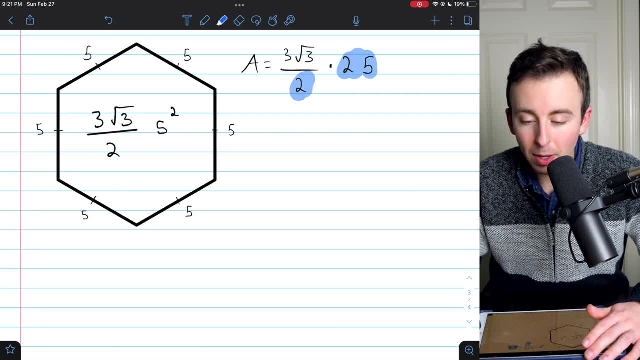 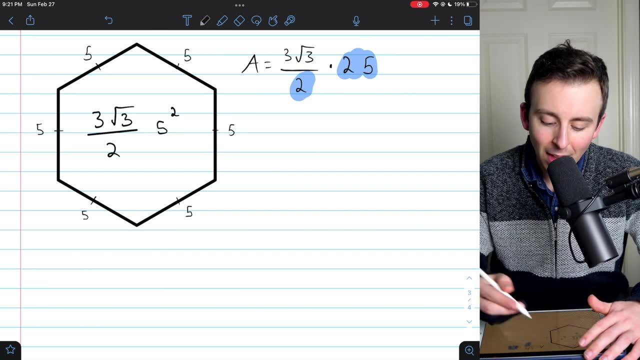 divide it by 2 nicely, like we did before. I mean, we could, if we want, and just use a decimal, But personally I like to keep things in nice cute looking fractions, So I'm going to go ahead and rewrite this as what. 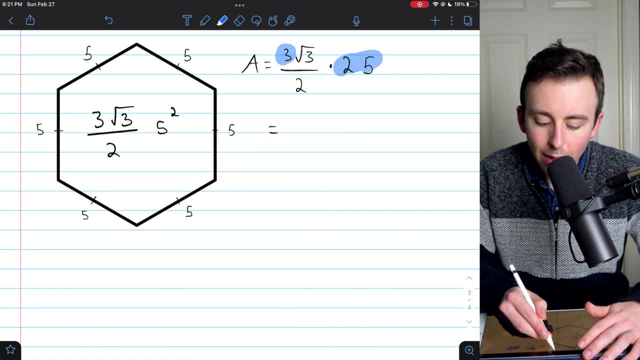 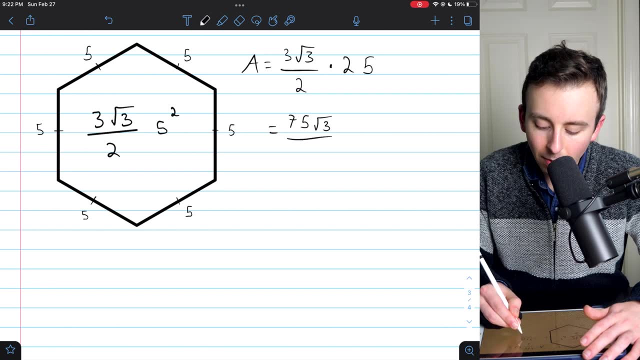 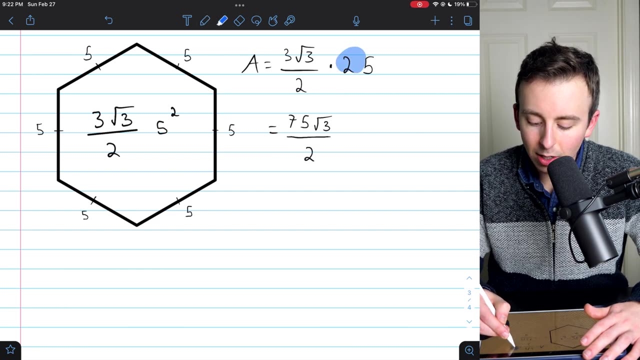 What Well, I'm just going to do 3 times 25.. So I'm bringing the 25 into the fraction and that's going to make this 75 root 3 over 2.. Let me rewrite that fraction bar 75 root 3 over 2, because we had 25 times 3 root 3 over 2.. 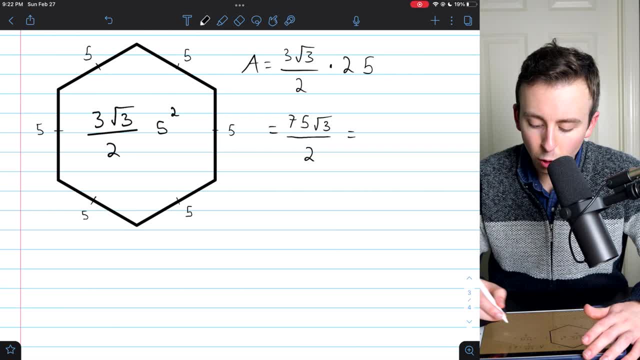 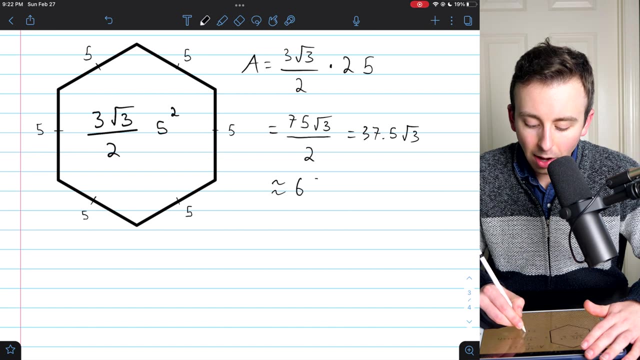 Now, if you like decimals, this is equal to 37.5 root 3.. That's just doing 75 divided by 2.. And then, if you want an approximation, this is approximately 65.. And you might just call it 65 units squared. 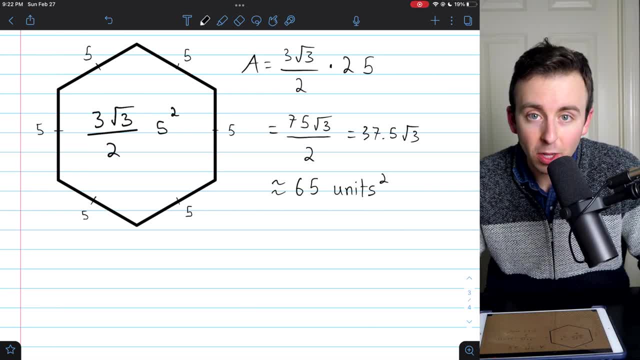 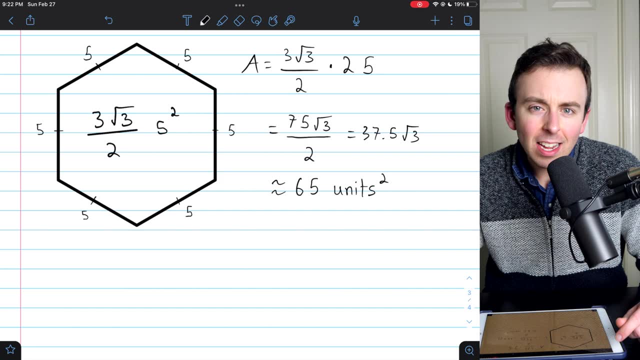 Whatever the units happen to be, area is a square unit, So we'll write it like that. That's all there is to it. That's how you find the area of a regular hexagon. Now let's take a minute to see where this formula comes from. 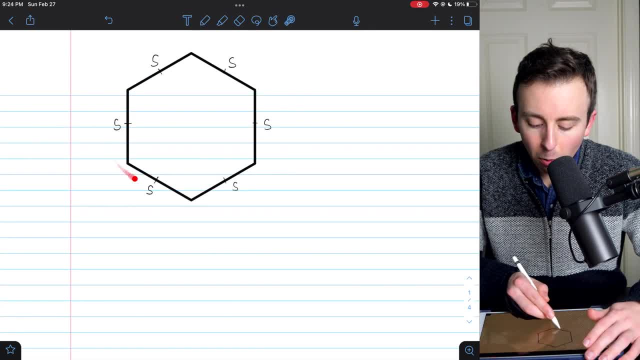 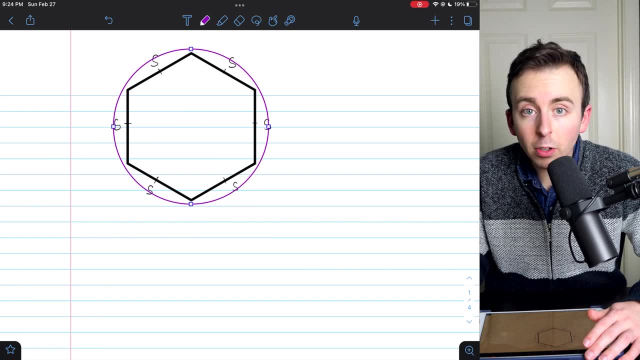 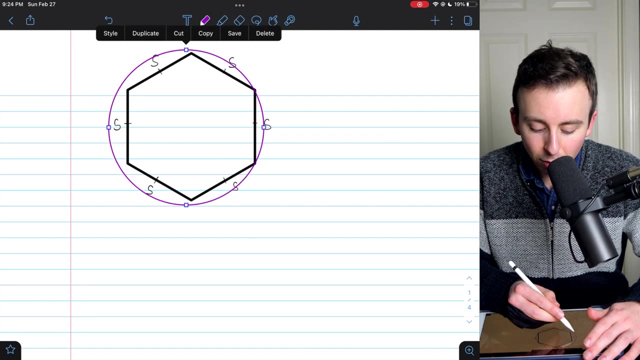 which really is the more interesting part Here, is our regular hexagon, And regular polygons like this have this cool property that we can draw a circle that circumscribes- That's what they call it. It circumscribes the polygon. That means this circle passes through every vertex of the regular hexagon. 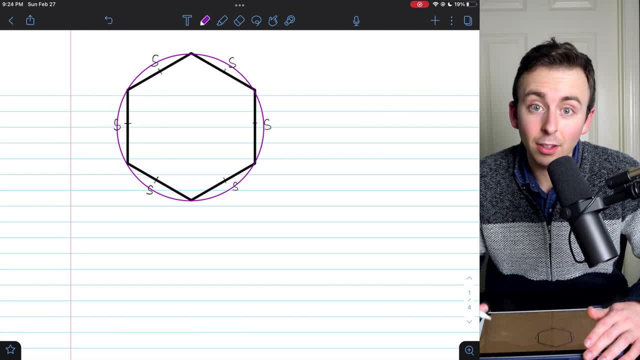 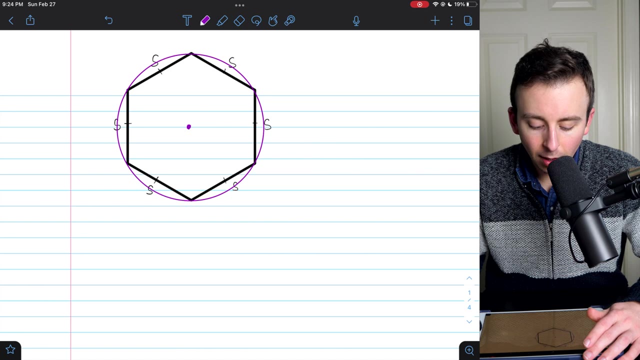 This is just a thing you can do with regular polygons. that's pretty cool. Now what I want you to imagine is that we've got this what's called a circumcircle passing through all vertices of the regular hexagon. Imagine we draw the center of the circle. 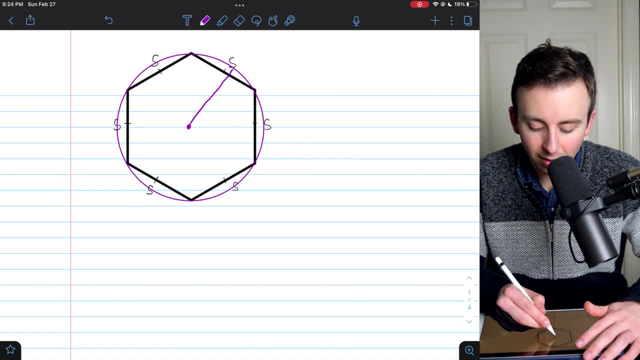 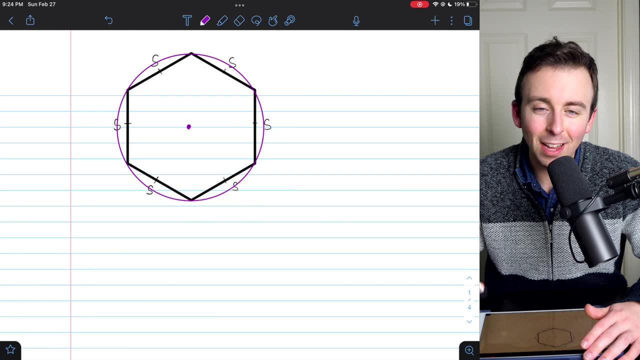 And of course there are radiuses that go from the center to the circle. I know the plural of radius is radii, but now you know that too, I'm going to say radii, Radii. There are all sorts of radii of this circle going from the center to the circle. 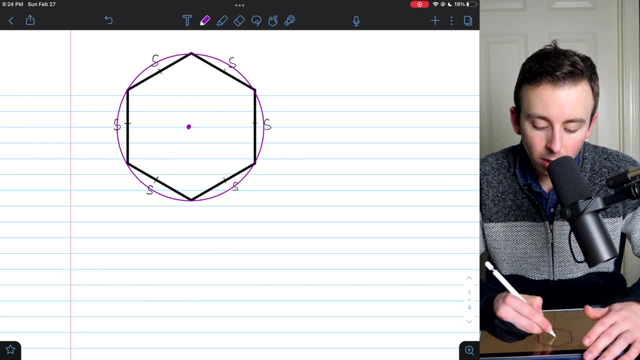 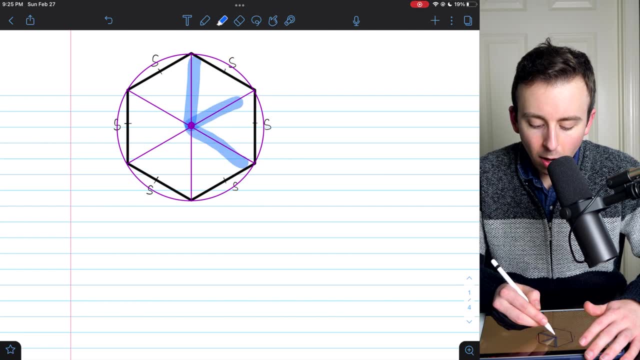 But let's draw the radii that go from the center to the center. They're going to be the vertices of the hexagon. I'm going to go ahead and draw those. This is what it looks like if we draw the radii from the center of the circle. 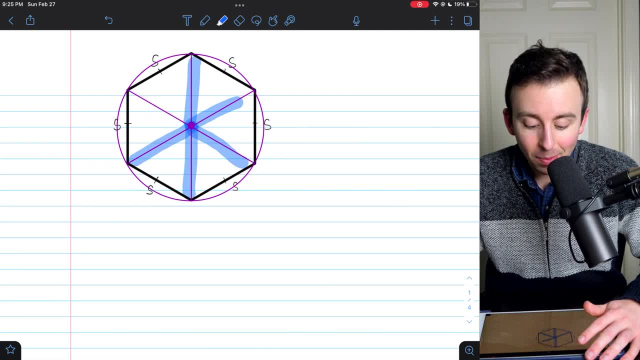 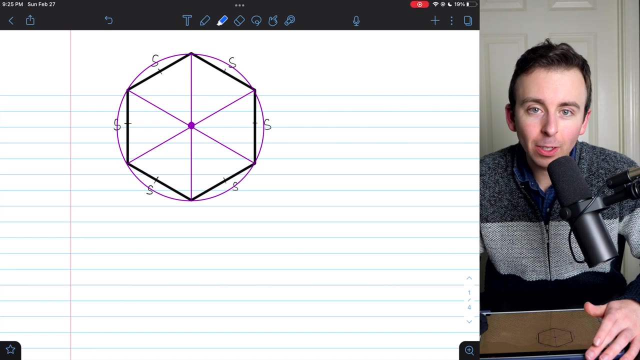 to the vertices of the hexagon And, you might notice, this splits the hexagon into six triangles. Now these triangles happen to all be congruent and regular, which means all of these triangles have side lengths that are all the same. We won't prove that in this video. 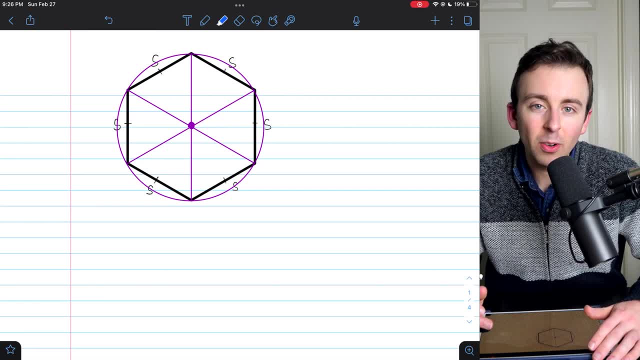 We'll prove it in a different video and I'll leave a link to that in the description. Definitely a really cool result that we can split a regular hexagon into six regular triangles. Now, if these triangles are all regular and congruent, 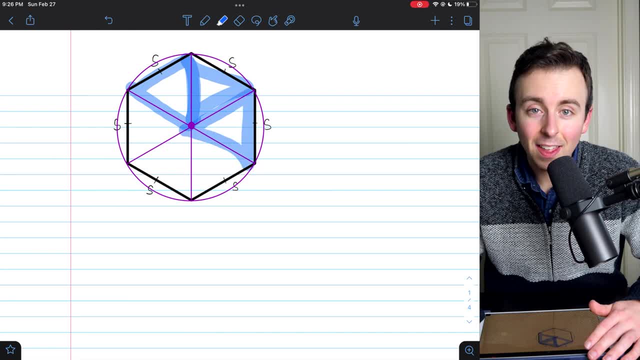 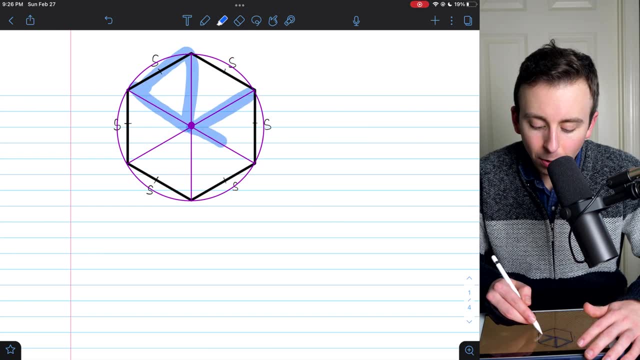 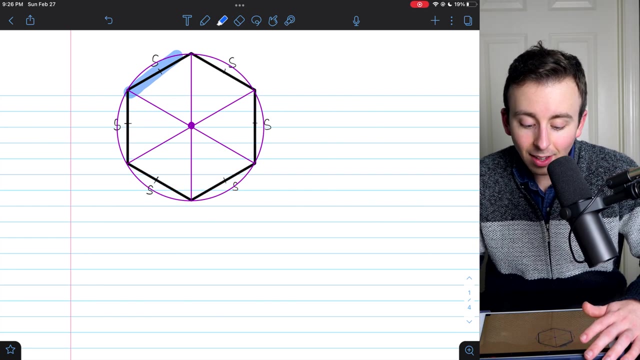 like I said, that means all their sides have the same length. But what is that length? Well, notice that each triangle has a side of the hexagon that is the same length. The hexagon has a side of the hexagon that is the same length as one of its sides. 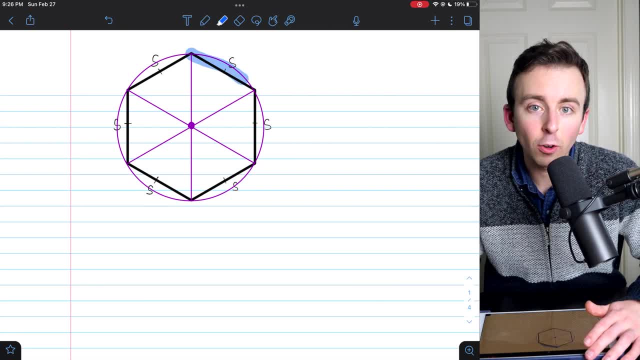 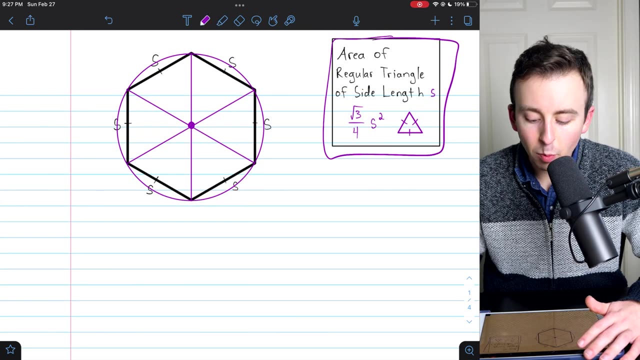 which means the sides of the triangles all have to have a length of s, just like the regular hexagon does. Now, it's pretty easy to calculate the area of a regular triangle, and it's from that formula that we get the area of a regular hexagon. 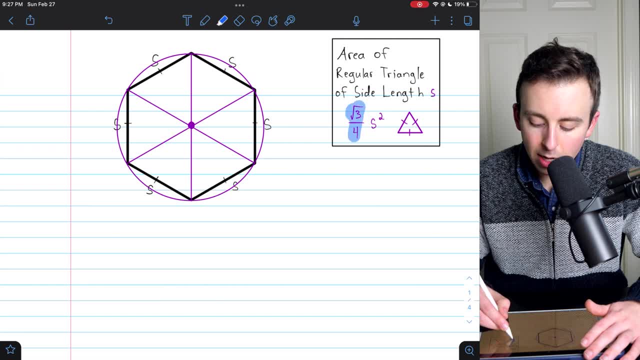 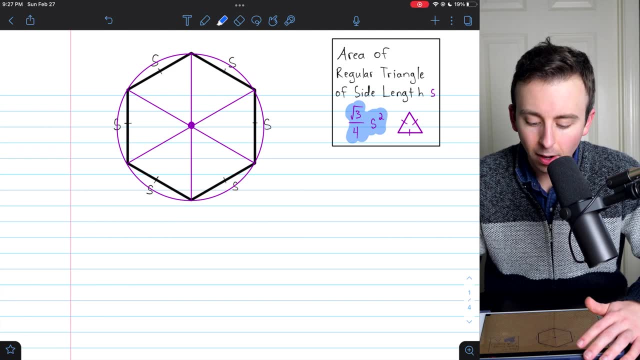 Right here is the area of a regular triangle of side length s. The area of a regular hexagon is s squared. So how do we take that and turn it into the area of our hexagon? Well, our hexagon just has six of these triangles. 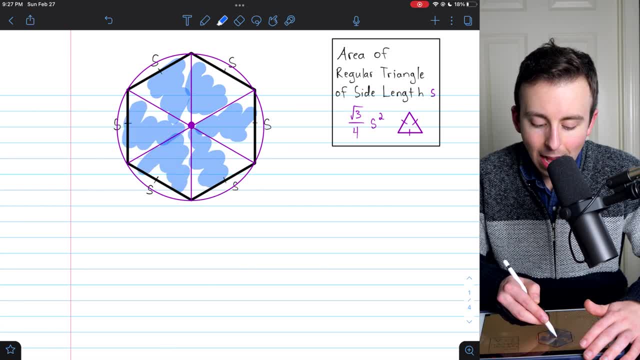 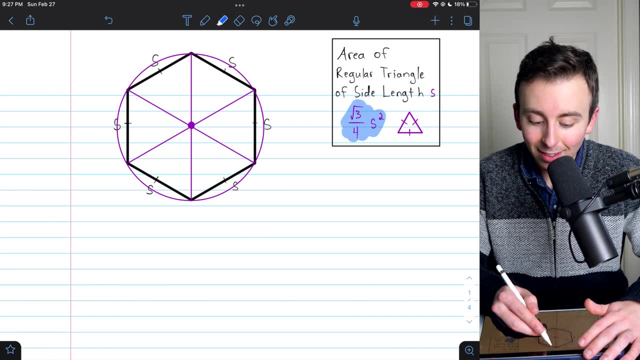 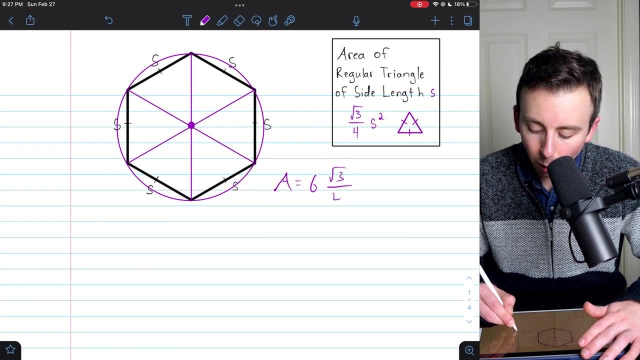 The six regular triangles make up the entire hexagon. So we just have to take the area of one of these triangles, which is given by this expression here, and multiply it by six. That gives us our area for a regular hexagon: It's six. 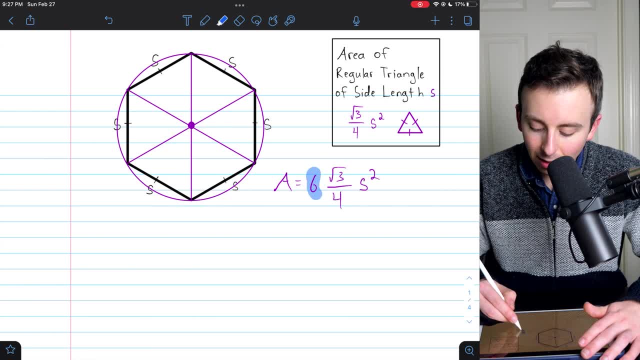 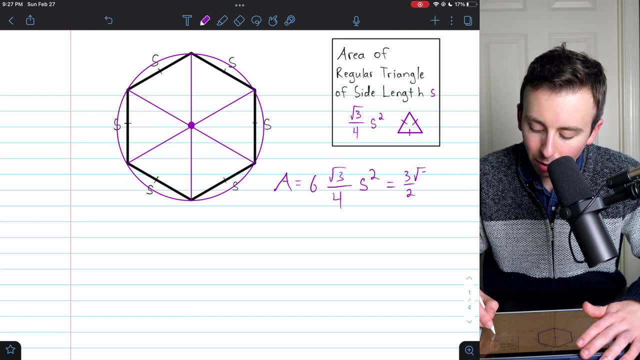 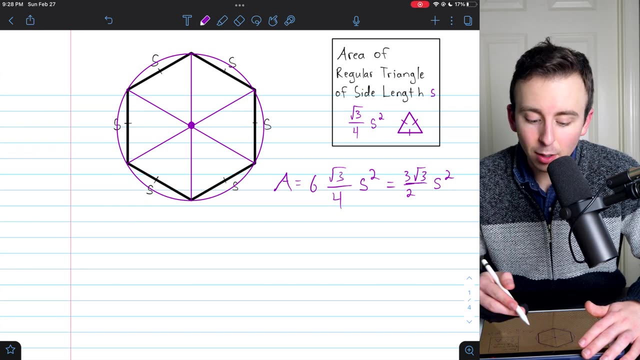 over four s squared and six over four. that's the same as three over two, giving way to the final formula that we've been using throughout this video, That's three root, three over two s squared, And I'll leave a link in the description to my lesson. 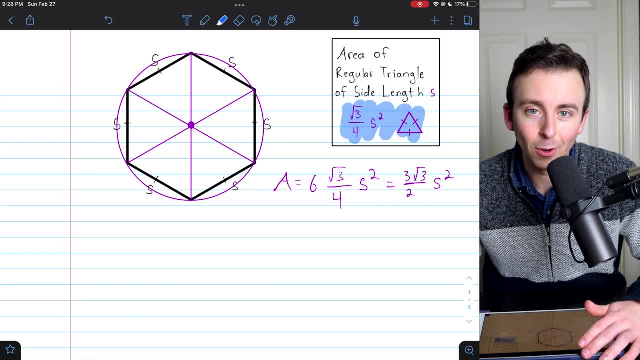 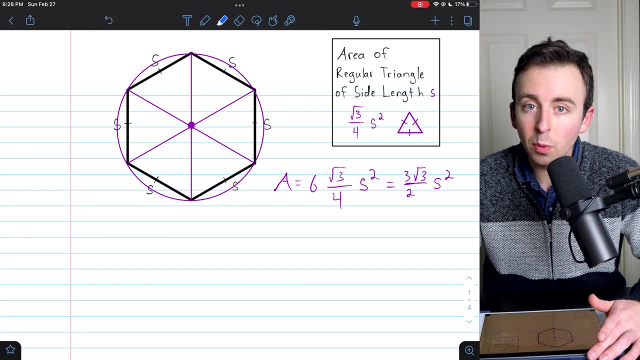 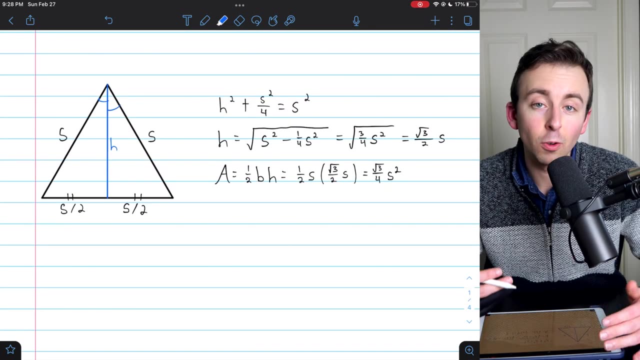 where we prove this area. formula for regular triangles. So that's where the formula for the area of a regular hexagon comes from. If you really want to have your curiosity fulfilled right now, here's a quick outline of the proof showing where the area of a regular triangle comes from. 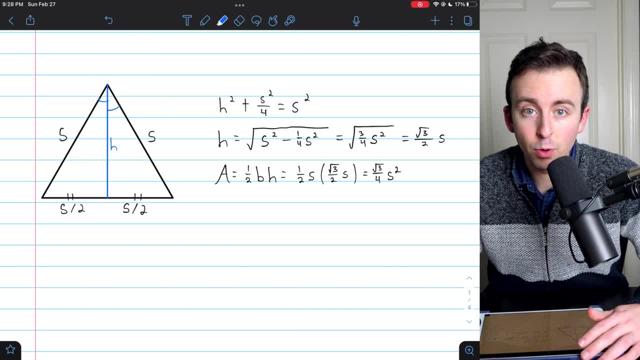 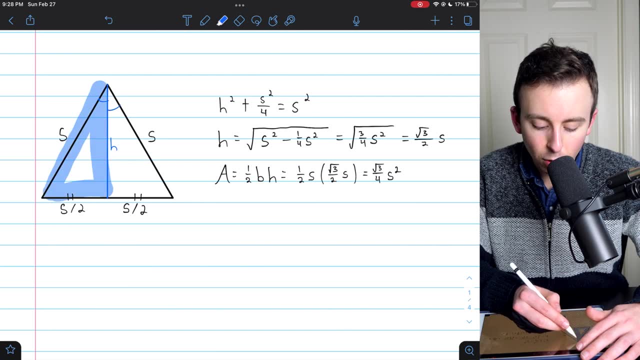 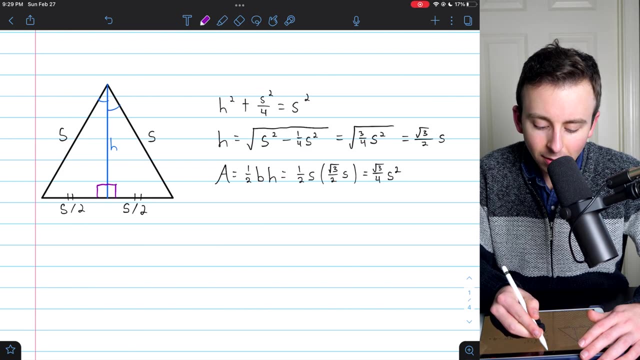 We just draw an angle bisector h through one vertex of the triangle and then, by side angle side, we've split it up into two congruent triangles, which thus means that these two angles are right angles and these two sides are congruent. 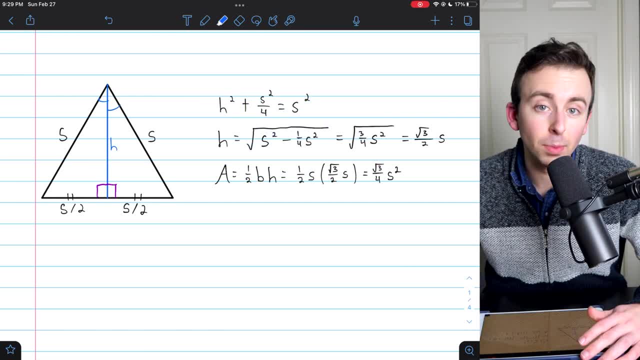 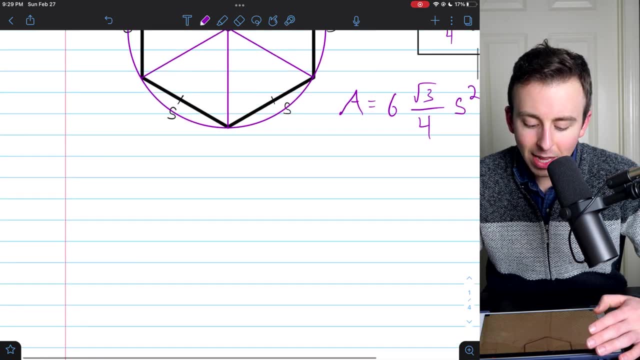 and then it just seems to me that we actually have consistent triangles of different angles, amounts to Pythagorean theorem and applying the familiar one half base times height formula for the area of a triangle. So that's it. That's how we calculate the area of a regular hexagon, and 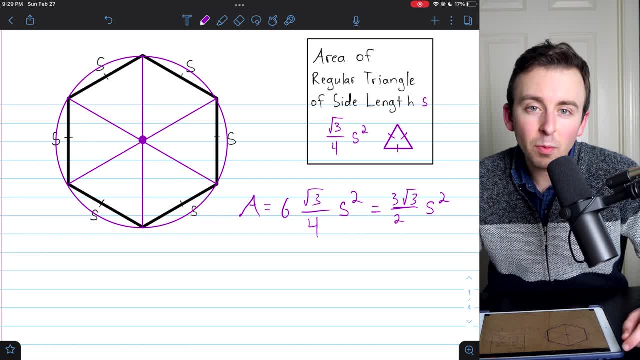 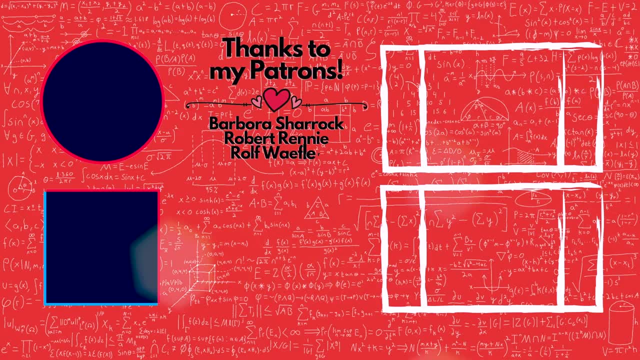 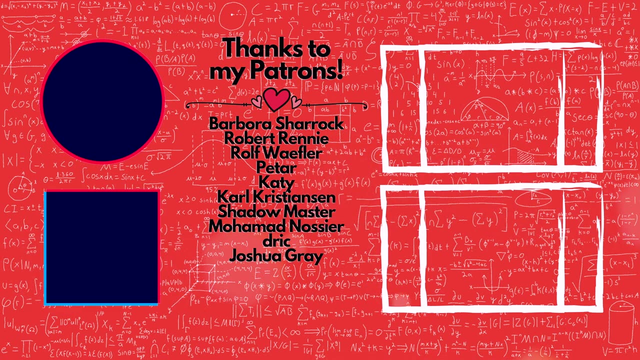 some details about where it comes from. Hope this lesson was helpful and let me know if you have any questions down in the comments. Thank you for watching.